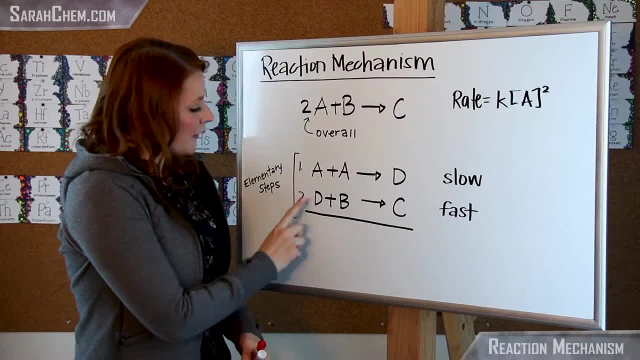 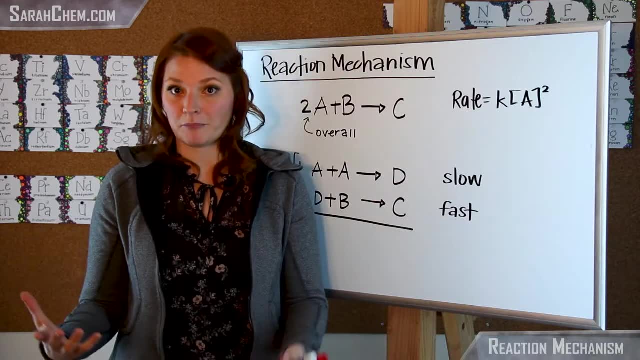 because D obviously doesn't appear here. The second step here has D react with B to form C. So these are the two steps that are required in order for the overall reaction to happen. So now there are a couple things you want to know about a reaction mechanism. The first: 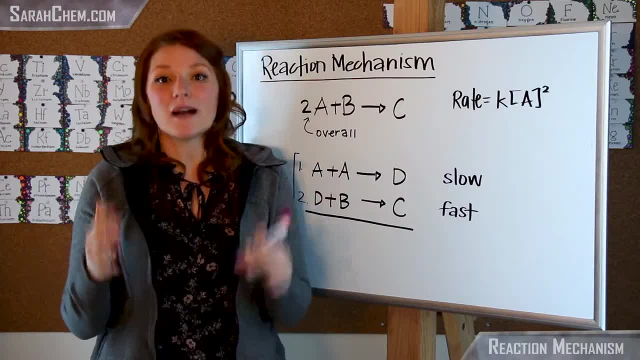 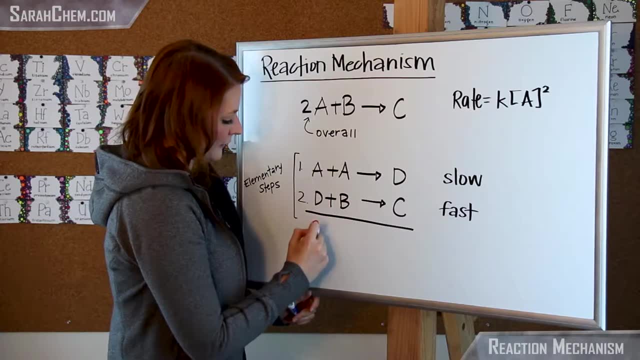 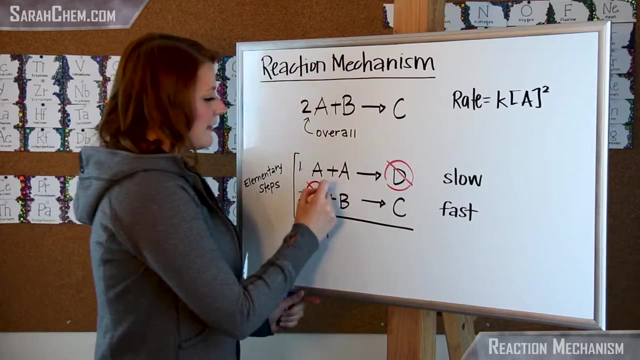 is when you add those elementary steps together, they must yield the overall reaction. So what I mean by that is this: If I take a look at this here I have 2As. Now you can see here D is a product and then D is a reactant. So that means it cancels out. 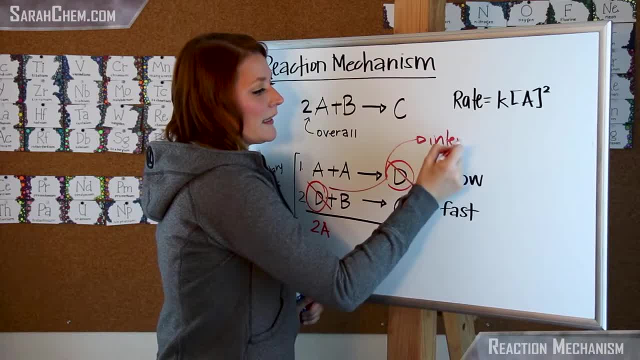 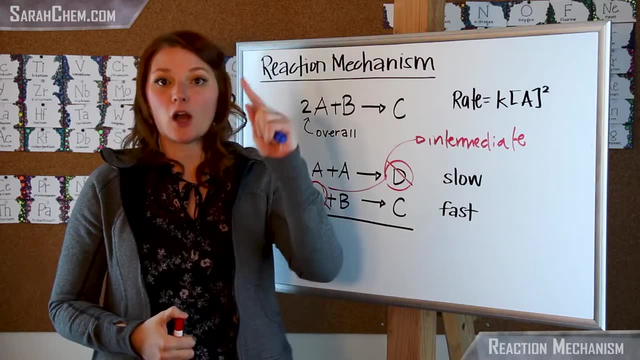 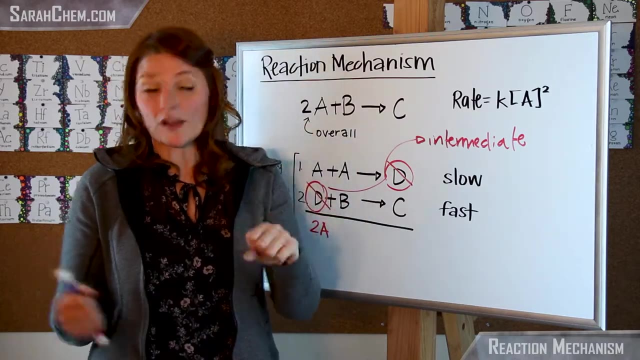 In the context of these, I would call D an intermediate. So an intermediate is some kind of species that is formed in the process of the reaction and then used. So it's going to start as a product and it's going to end as a reactant and it will cancel out. It is. 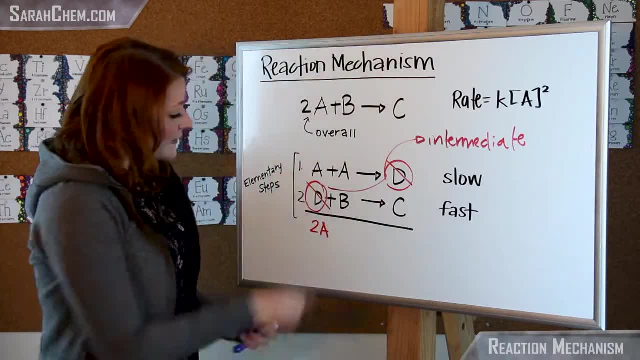 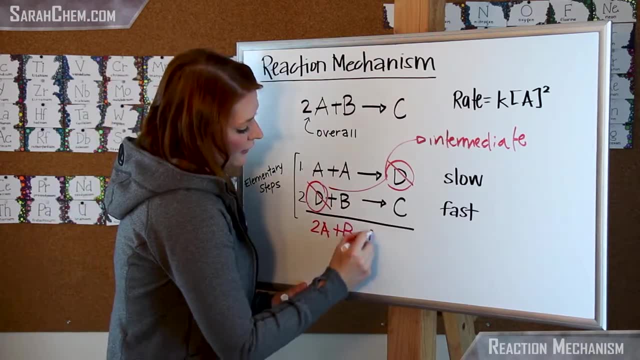 not going to be present in the overall reaction. So that means there will be no D in this overall reaction. as I'm adding these two together, Then I say I have one B and they will form a C. So you can see that this reaction and this reaction are equivalent with one another. 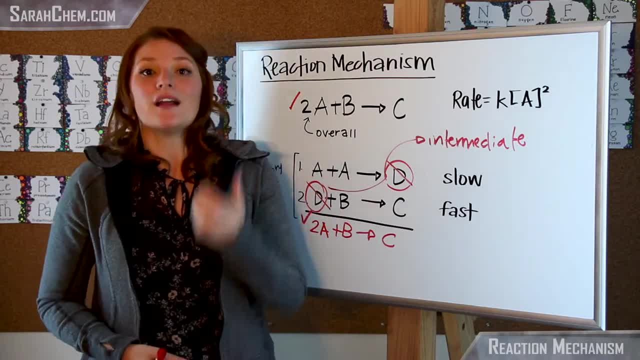 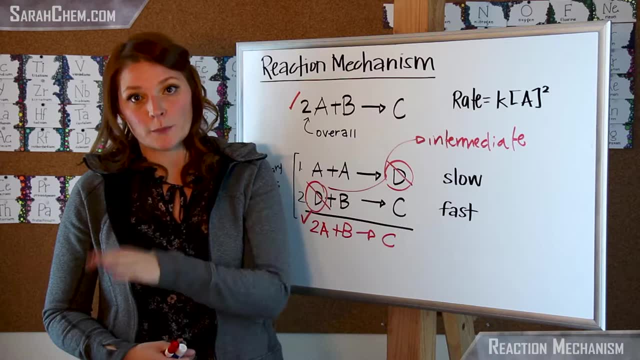 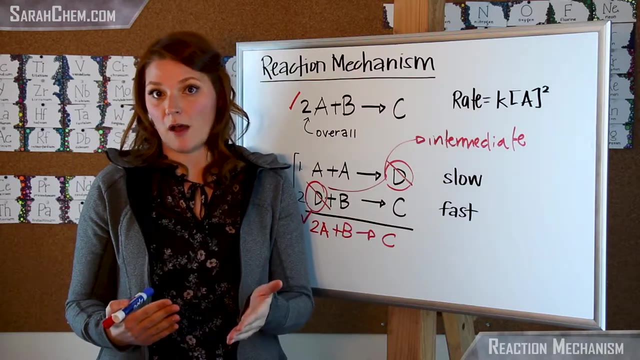 So that means that my reaction mechanism passes the first step. The next thing is that the rate law of my reaction mechanism has to be equivalent to the experimentally determined rate law. So you do an experiment to figure out what a rate law is, and the mechanism that I put forth has to have a matching rate law. Now what's? 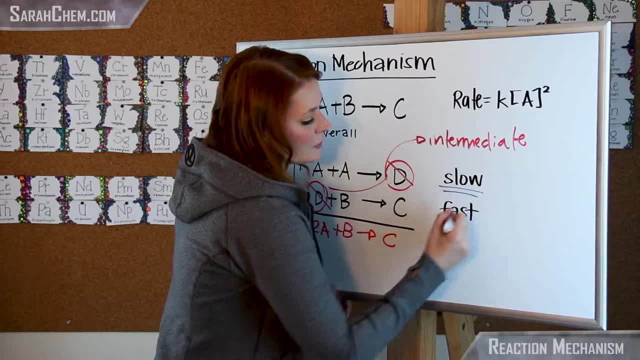 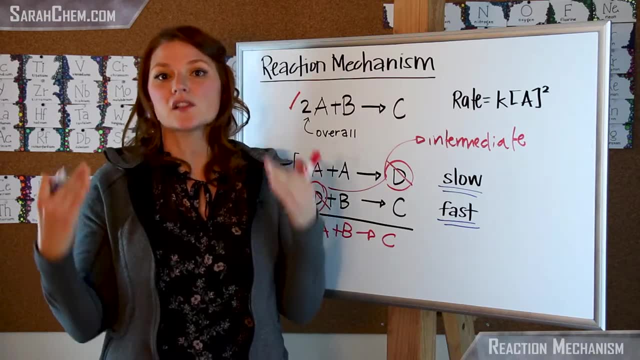 going to be important when you're talking about that is these words here: slow and fast. So we have something called a rate determining step. The rate determining step is the same as the slowest step in your mechanism. Your reaction can only go as fast as the slowest. 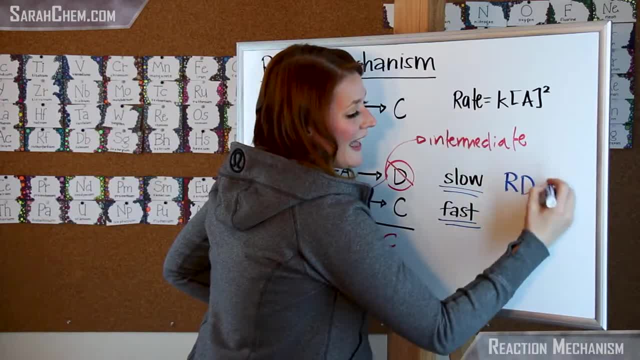 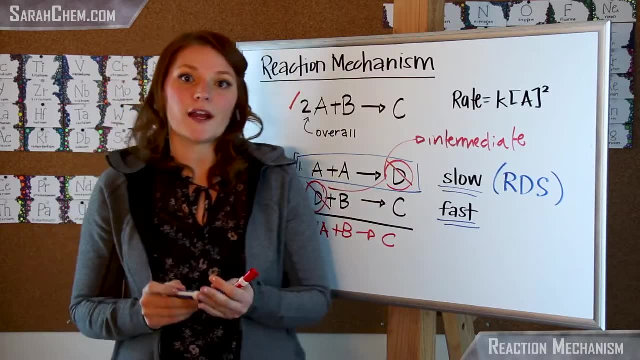 component, So this one here we're going to abbreviate RDS for rate determining step. So that means that I'm going to use the first elementary step in order to figure out what the rate is according to my reaction mechanism. Keep in mind that my rate law is a little bit more complex. I'm going to give you a 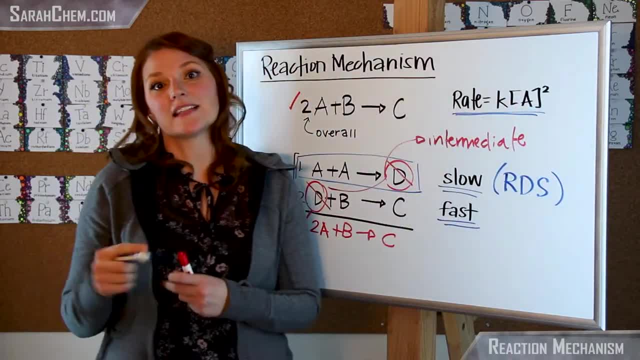 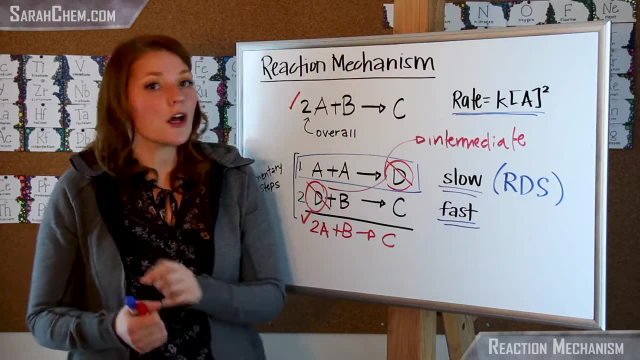 my one that I've determined experimentally, is: the rate is equal to k times a squared. So now a few things. Remember that when you're talking about a rate law, you cannot use the coefficients in the overall balanced equation to figure out what the rate law is Right.